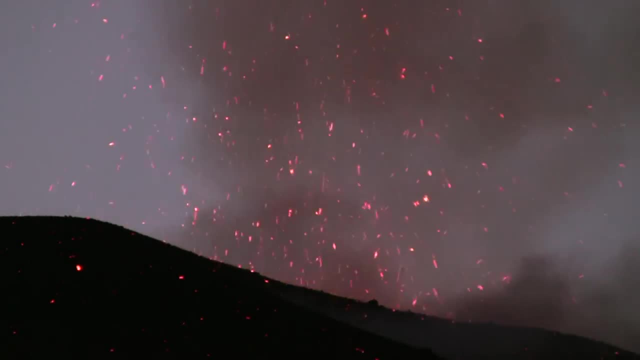 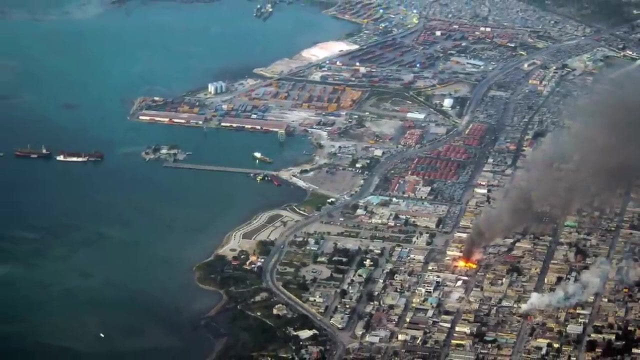 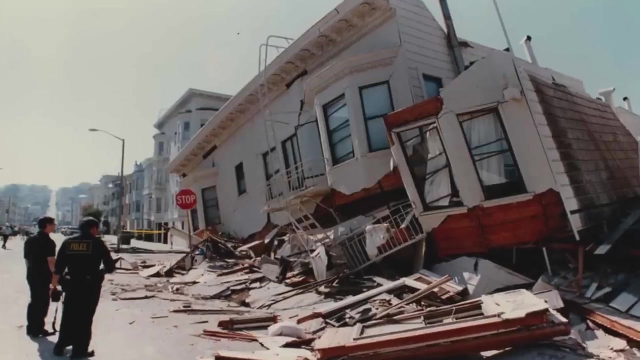 may erupt following a series of earthquakes. In 1989, the monstrous earthquake of the Bay Area in California rocked the major cities of San Francisco and Oakland. The temblor caused landslides, fires, buildings crumbled and cracked, homes demolished, A double-decker freeway collapsed. 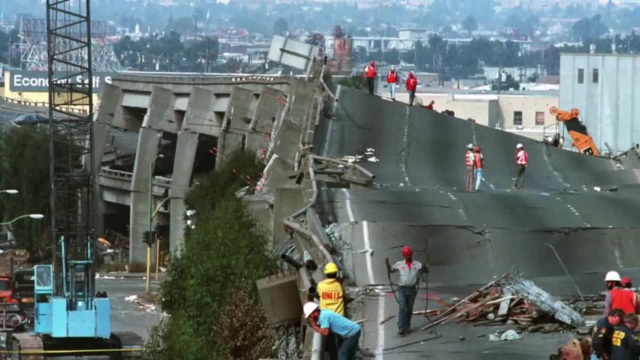 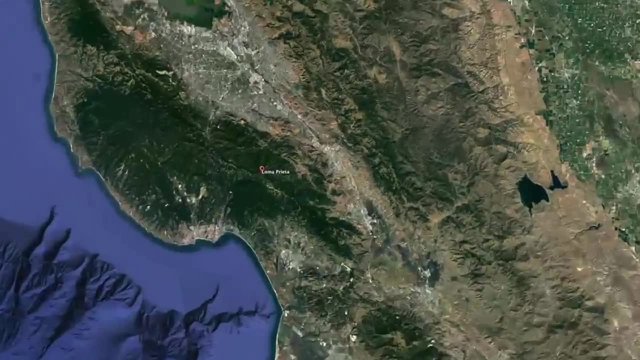 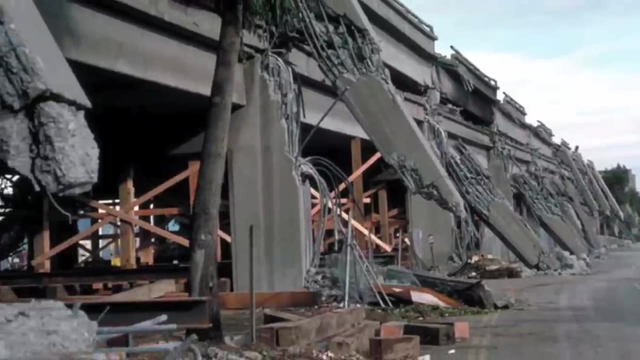 and flattened cars below. The damage came to a cost of billions of dollars to repair. The epicenter where the greatest forest originates was 60 miles away, And yet these two major cities were struck with enormous force and destruction. There were fewer cars than usual during rush hour on the 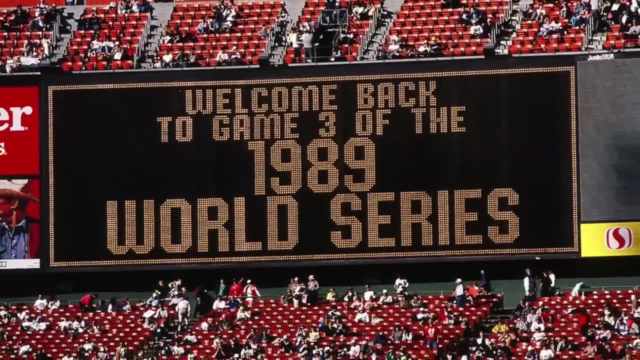 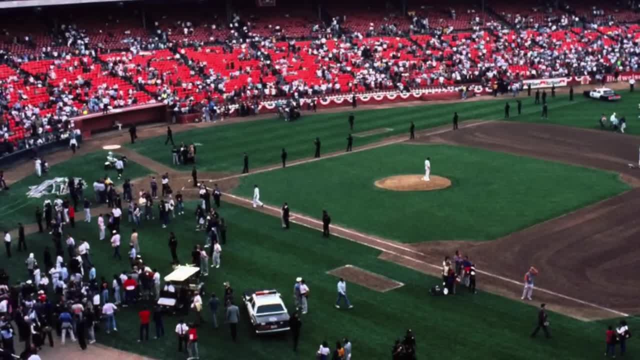 roads and expressways. You see, on that day, October 17, 1989, Game 3 of the World Series was being played in San Francisco's Candlestick Park. The Oakland A's and the San Francisco Giants and their fans were in the stadium when the earth shook. 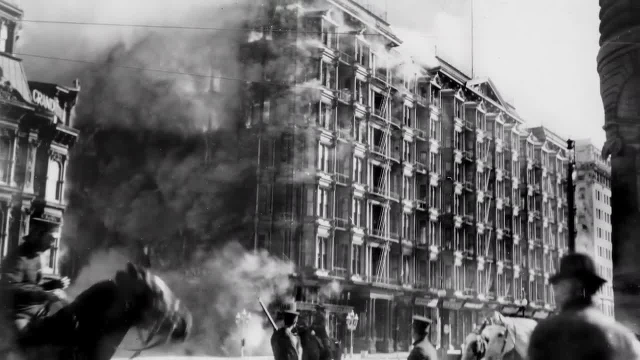 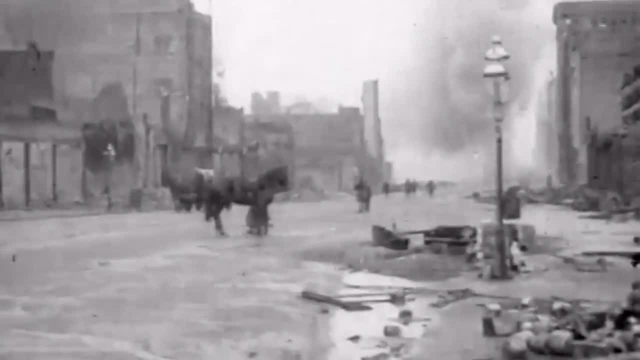 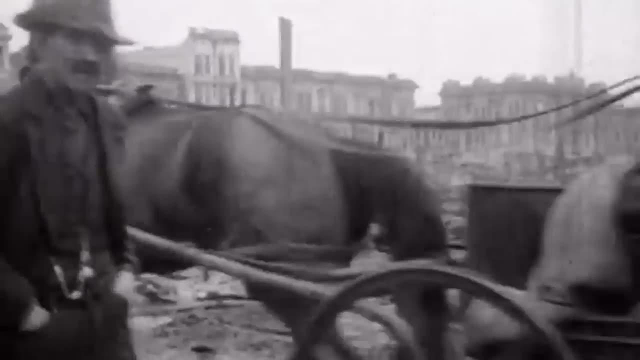 Amazing. Even more shocking: San Francisco was also the site of the devastating quake of 1903. At that time, the entire city was mostly destroyed. Throughout history, millions of people have been affected by the wrath of the invisible destroyer. You don't see it coming and you may not know when. 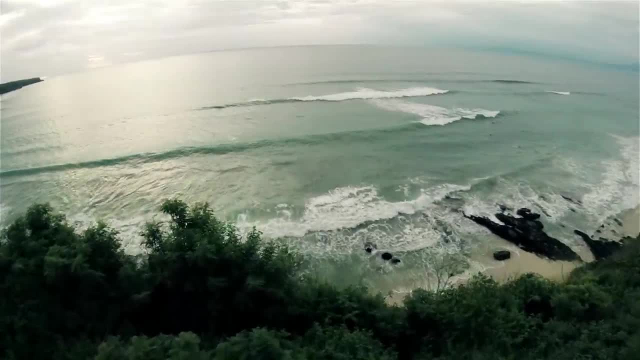 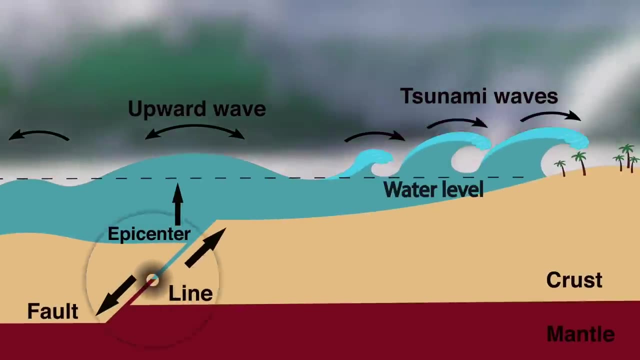 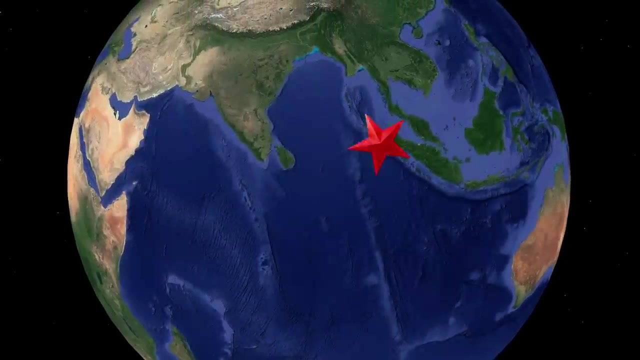 it will strike The day after Christmas of 2004,. many miles below the seabed of the Indian Ocean, the movement of two tectonic plates caused a series of enormous waves of water, over 100 feet high, to strike 14 countries bordering the. 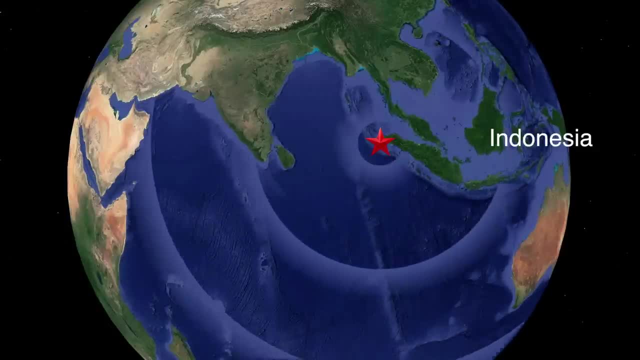 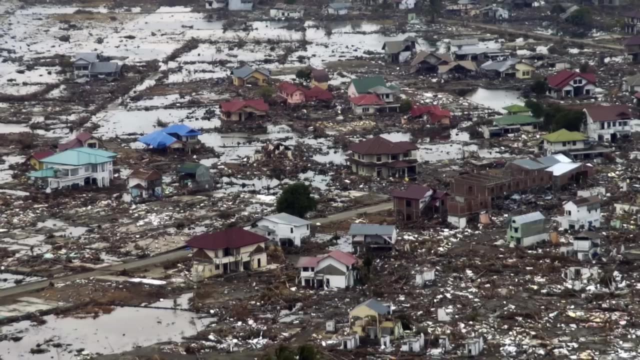 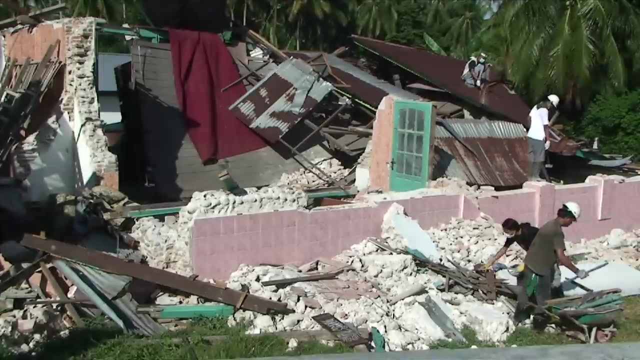 Indian Ocean. Indonesia was the hardest hit, then Sri Lanka, India and then Thailand. Hundreds of thousands of people were affected. These huge waves caused by earthquakes are named tsunamis. Any coastal town is at risk of being struck by a tsunami. They can begin from hundreds of miles out. 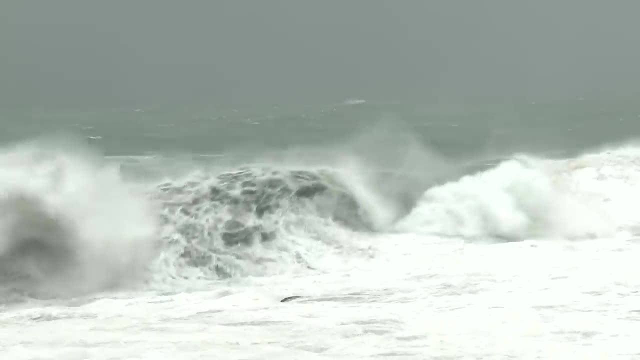 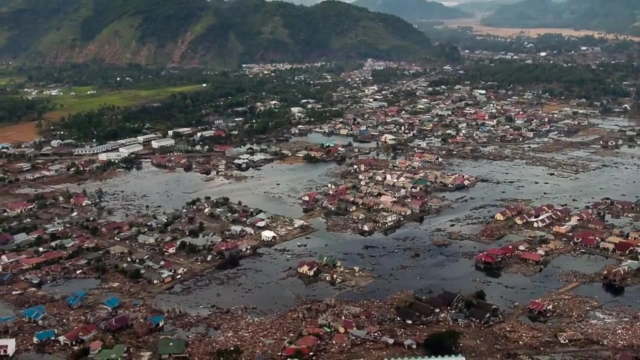 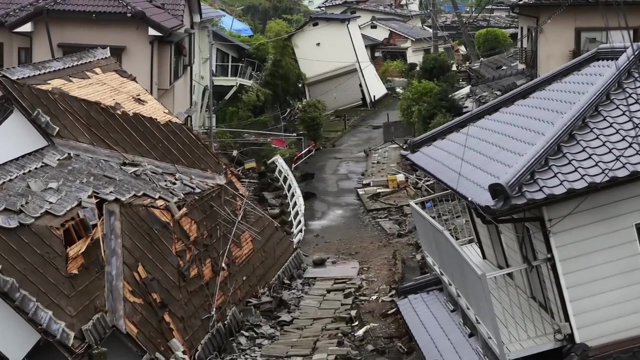 and travel at a speed of over 500 miles an hour- As fast as a jet. You cannot outrun, outdrive a tsunami. The wall of water may travel for miles and miles inland and the best thing to do is head for higher ground. If you should be caught in an earthquake, there are some things you can do.